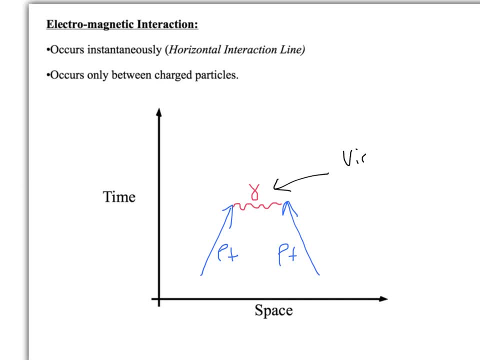 So Let's just quickly label that in there, Okay. So key things you should know about a virtual photon is: it has zero rest mass And it has zero charge. So there's a couple of key points there. So, coming out of it, what do you have? 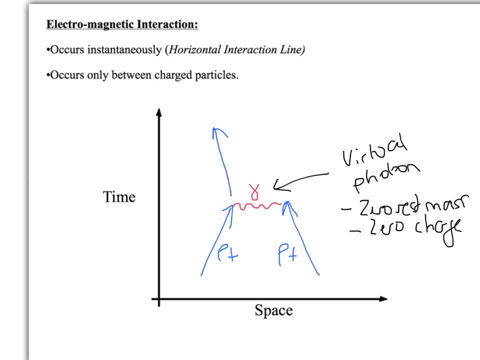 Well, electromagnetic interaction doesn't actually change, It just obviously has an effect on them. So you'd still get two positively charged protons leaving, But obviously they would have exchanged the virtual photon, which is like a force carrier. 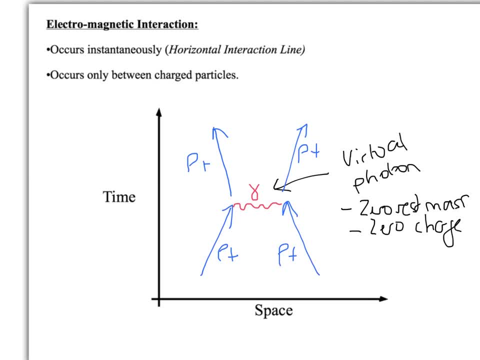 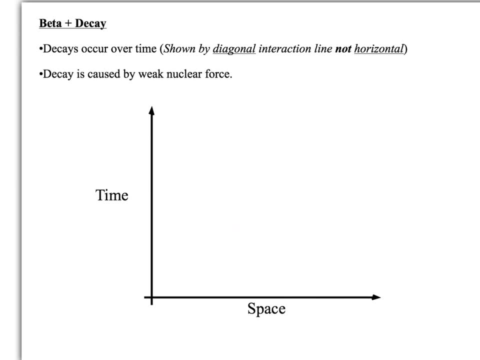 So they've had a slight repulsion. So you'll see them angled away, just like on this diagram. Okay, So let's have a look at another example. This is beta plus decay. Now, decay is caused by the weak nuclear force. 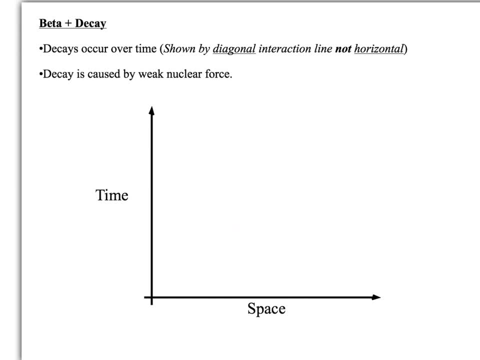 So obviously a beta particle. What we'll use for beta plus is actually going to be a proton, So we have our proton coming in just as before. So protons are obviously a type of hadron, So they don't interact through the weak nuclear force. 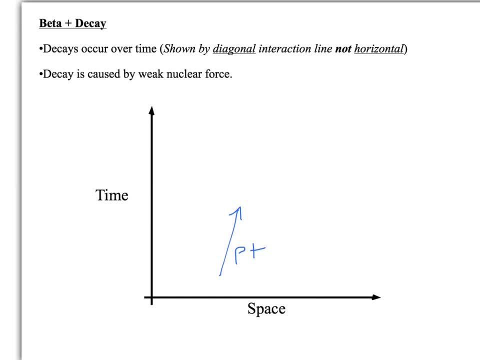 They decay through the weak nuclear force, And protons are made up of just a little bit of extra information- up, up, down quarks, And weak interaction causes one of these to change into another one. So one of these up quarks is actually going to become a down quark. 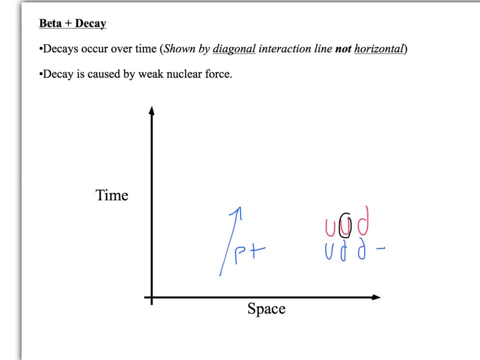 So now it becomes up, down, down, which is a neutron. Okay, So what we have coming out of it is a neutron which obviously has no charge. So one of the key properties in the universe: charge in all types of interaction. 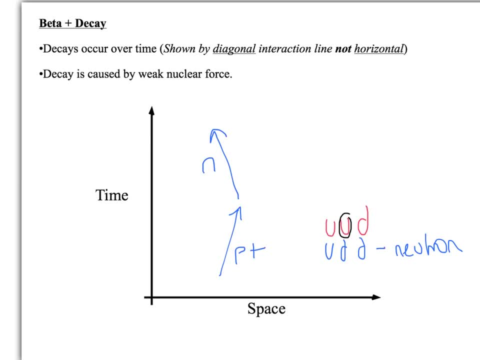 and reactions and stuff charge is conserved. So there must be another particle coming off which carries that charge so that charge is conserved because it's plus one at the start and obviously it needs to be plus one at the end. 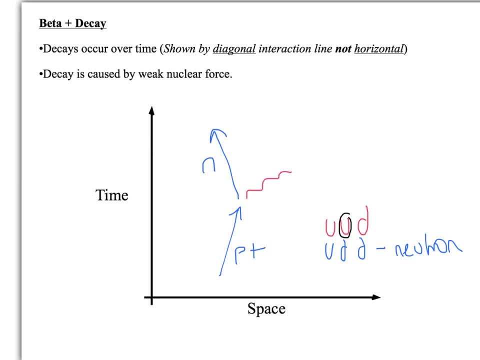 So when we do our interaction line, this time you must be giving off a charged particle and it must be positively charged, which means it's your W plus boson. So this interaction decay occurs over time, Which is why the interaction line is angled slightly up to show the passage of time. 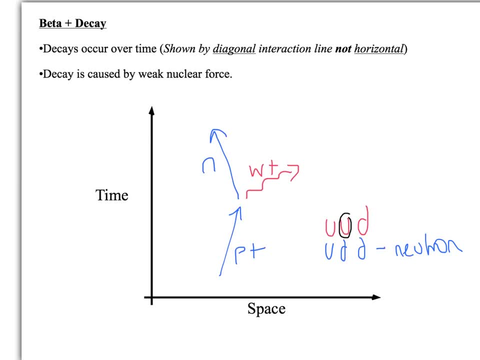 So what happens next? Well, the W plus boson itself decays into two particles, So it forms a E plus, or it's often called a beta plus particle, And also in terms of that you get a neutrino being. 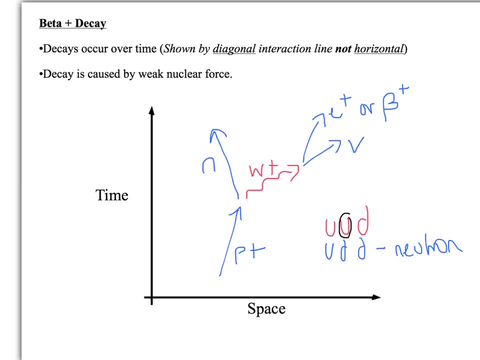 formed due to the conservation laws which I talk about in another video. So that's a Feynman diagram for beta plus decay. So you can see, a decay occurs over time and that's why the interaction line is angled upwards.